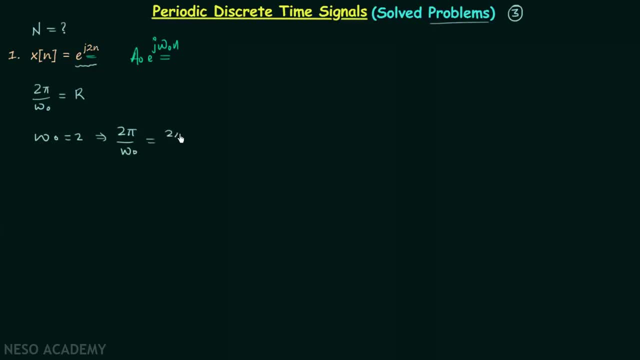 by omega0 is equal to 2pi divided by 2. And we will finally have pi, And pi is an irrational, irrational number. This is an irrational number and therefore the given signal, xn, which is equal to e power, j2n, is non-periodic. So this is the answer: The given signal is non-periodic. 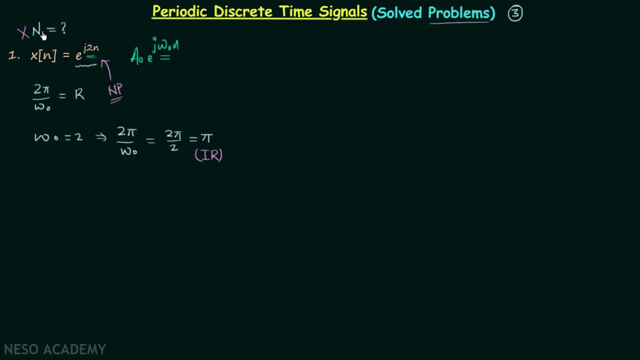 and therefore the period will not exist. Now we will move on to the second problem. In the second problem the discrete time signal xn is equal to cos 3pi by 4n. So here in this case we are having a sinusoidal discrete time signal and, like discrete, complex exponential 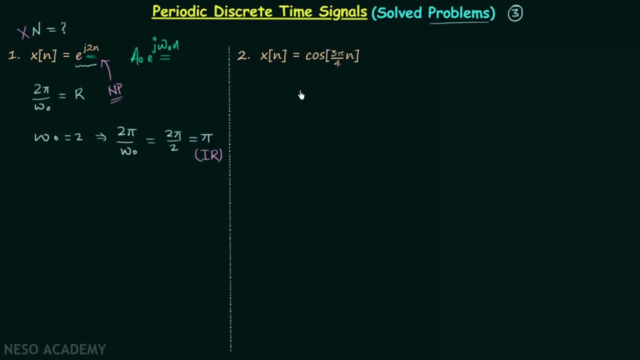 signal. discrete sinusoidal signal may or may not be periodic. Again, this condition must be satisfied. So Omega naught in this case is equal to 3pi divided by 0. 4, 3 pi divided by 4, and now we will check whether 2 pi divided by omega naught is giving. 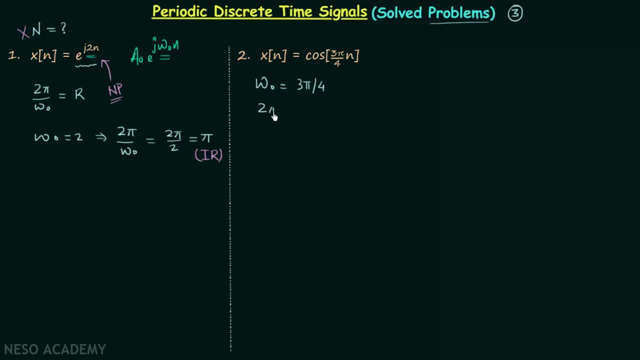 us a rational number or not? So let's divide 2 pi by omega naught, which is 2 pi divided by 3 pi divided by 4, 3 pi divided by 4, and this is equal to 8 divided by 3.. 8 divided. 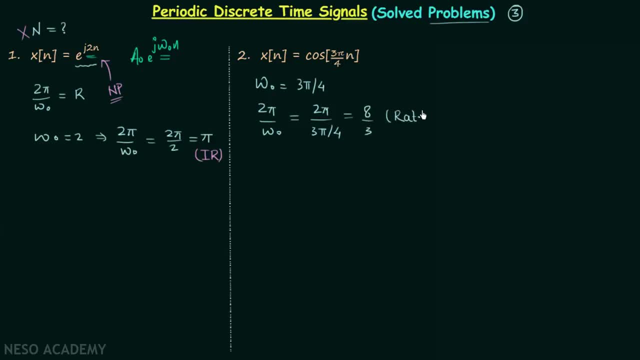 by 3 is rational and therefore this signal is periodic. This signal is periodic and therefore we will calculate the period n, and we know 2 pi divided by omega naught is equal to n divided by k. This implies period n is equal to 2 pi divided by omega naught multiplied. 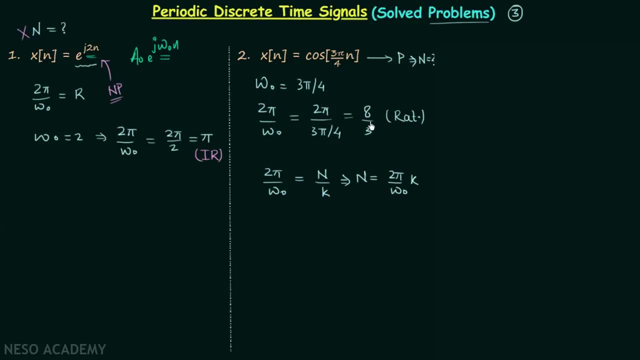 to k. 2 pi divided by omega naught is equal to 8 by 3.. So n is equal to 8 by 3 multiplied to k. and we know the fact that n is an integer and to get an integer value, k must be equal. 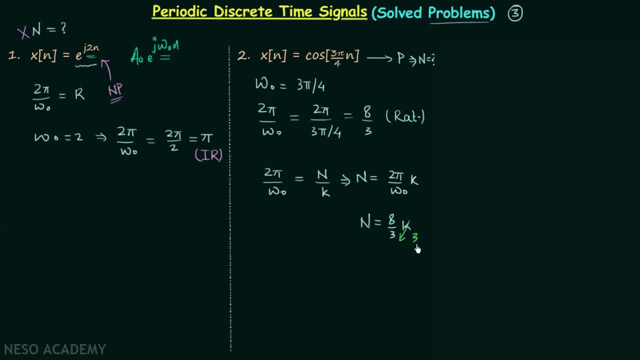 to 3.. Taking the minimum value of k, it should be 3 and therefore we will get the period, which is a fundamental period, equal to 8.. So this is our answer. You can also consider k equal to 6.. When you consider k equal to 6,, you will have n equal to 8 by 3, multiplied by. 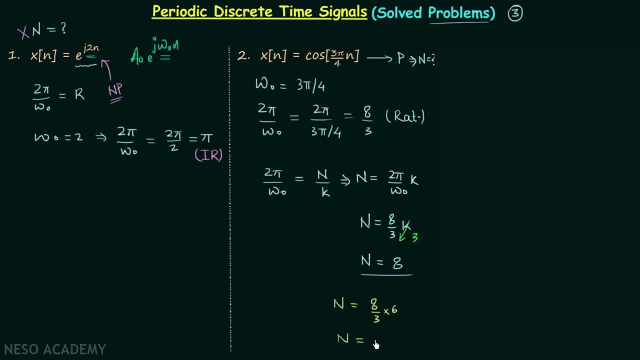 6, which, in tons, give you n equal to 16.. But 16 is not a fundamental time period, It is simply the period. It is equal to 2 times the fundamental time period 8.. So this is the answer, and we usually represent the fundamental time period by: 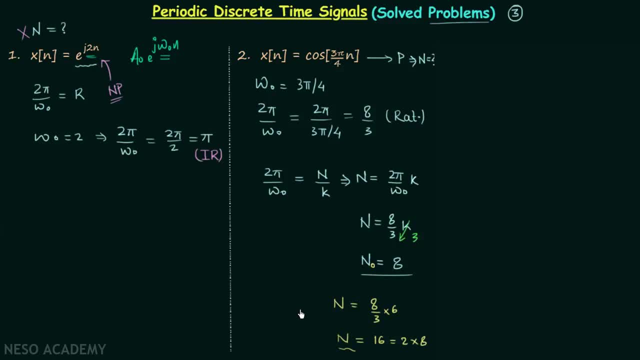 n, subscript 0. So we can say that this period n is equal to two times the fundamental period n0.. Similarly, you can consider the other values of k as well. For example, when you consider k equal to 9, then you will have the period equal to three times. 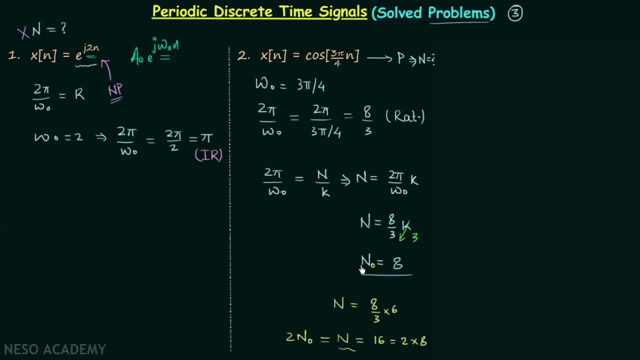 the fundamental period n0.. But in question you are required to calculate the fundamental period, which is 8.. Now we will move on to the third and the last problem, and here we have a composite discrete time signal. Xn is a composite discrete time signal. 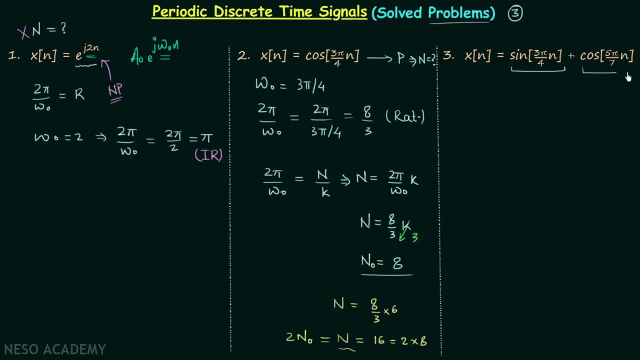 It is equal to this signal plus this signal, and let's say this signal is X1n and this signal here is X2n. and if you see signal X1n you will find 3 pi by 4 is equal to omega 0 and we have already calculated the fundamental period when omega 0 is equal. 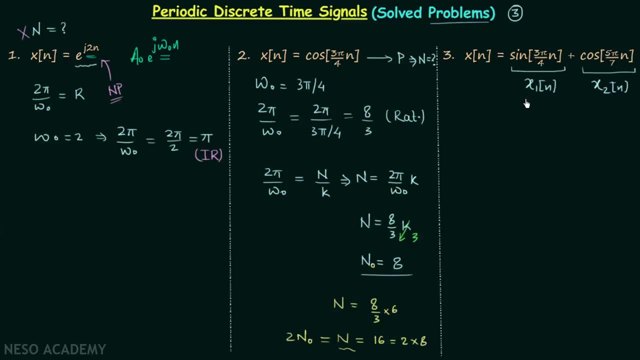 to 3 pi by 4 and therefore for this signal we will get the fundamental period- let's call it n1- equal to 8.. Now we will focus on this signal, X2n, and in this case we are having omega 0 equal to 5 pi by 7.. 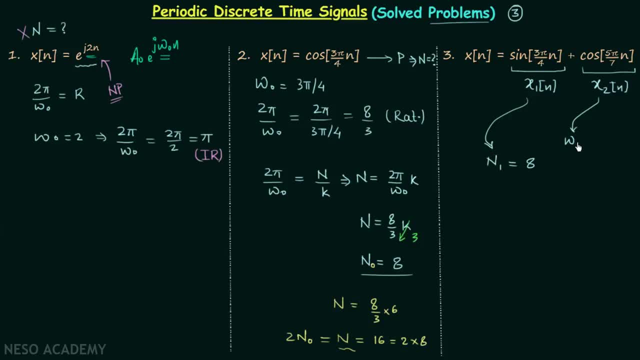 So omega 0 we are getting as 5 pi by 7. and first we will check whether this sinusoidal signal, which is a discrete sinusoidal signal, is periodic or not, and for that we will check whether 2 pi divided by omega 0. 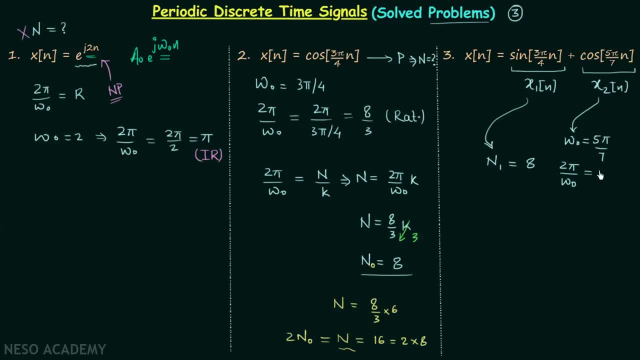 is giving us rational value or irrational value. Now let's see whether 2 pi divided by omega 0 is giving us rational value or irrational value. So, for example, if we were to find a sine signal of pi which is at least 2 pi divided by omega 0. 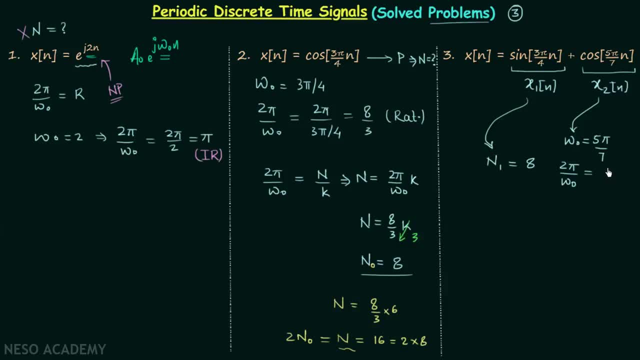 2 pi divided by omega naught, which means 2 pi divided by 5 pi divided by 7, will give you 14 divided by 5, which is definitely a rational number. This implies the signal we are having here is a periodic signal. 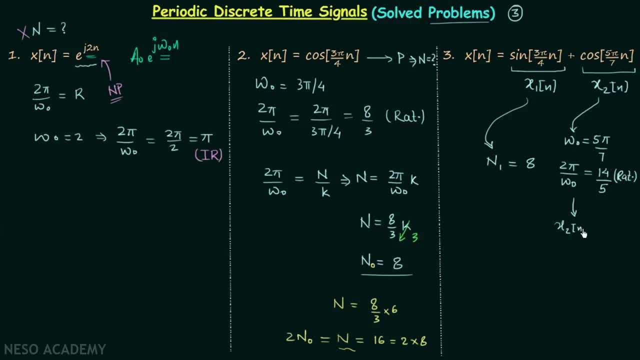 The signal we are having, which is x2n, is a periodic signal and therefore we will calculate the period n. n is equal to 2 pi divided by omega naught multiplied to k. 2 pi divided by omega naught is equal to 14 divided by 5 multiplied to k. 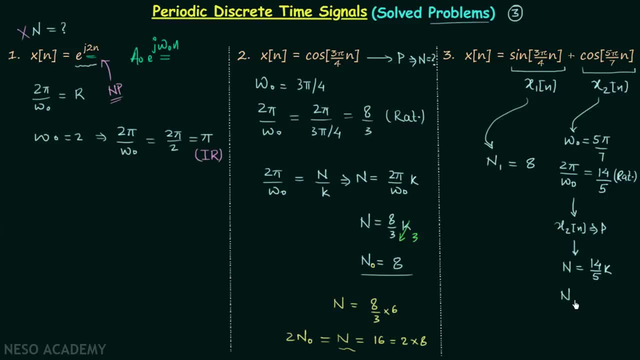 For fundamental time period. let's call n2, k must be equal to 5.. In that scenario, we will get the integer value of n2 and only integer values are valid for the period. Therefore, 14 is the fundamental time period of this signal. 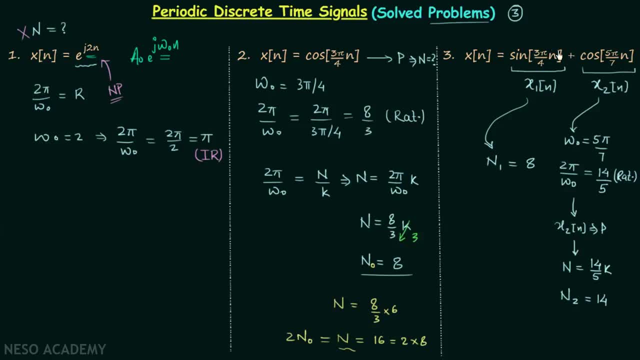 So we have obtained the fundamental time period of this signal equal to 8, and fundamental period of this signal equal to 14.. And our aim is to calculate the fundamental period of signal. So do try to calculate the entire period of barking signal xn, which is the composite signal. 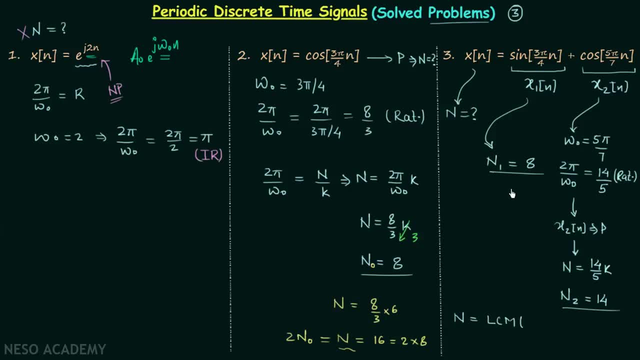 And in the previous lecture I told you, calculate n. simply calculate LCM of n1 and n2.. This means LCM of 8 and 14. And when you solve it you will get 56. So the fundamental time period of this composite signal is equal to 56.. 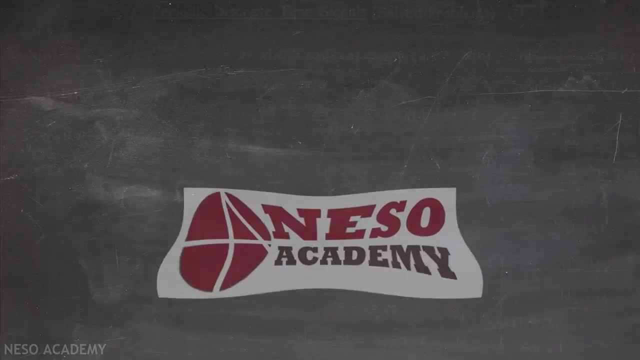 And this is mg. This is the answer.